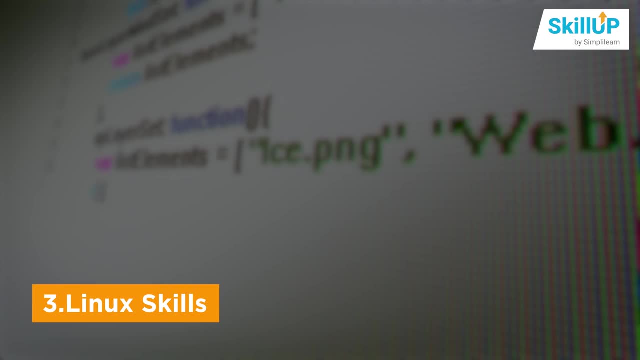 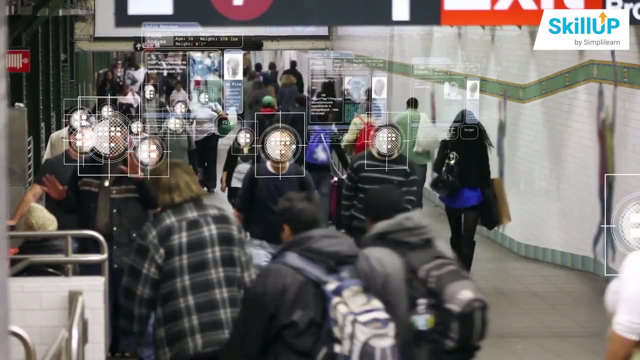 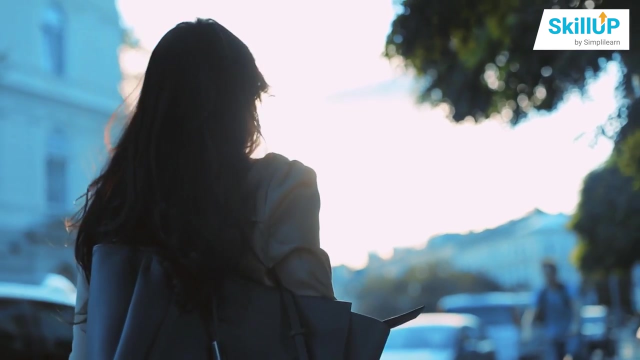 After polishing your networking skills, the third obstacle should be getting your knowledge of Linux operating systems to above average standards. Most scanning tools and exploit frameworks run exclusively on Linux-based distributions like Kali Linux and Parrot Security, making it an absolute must, before moving forward, A course on the basic introduction to 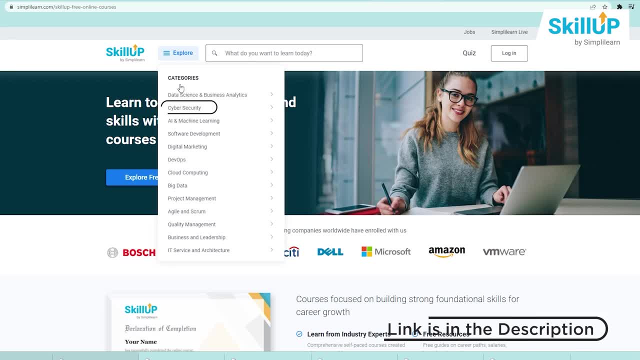 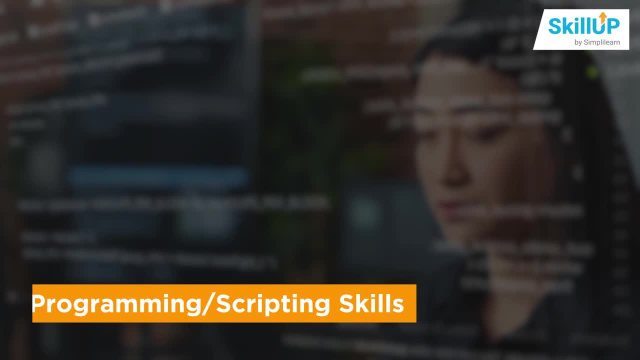 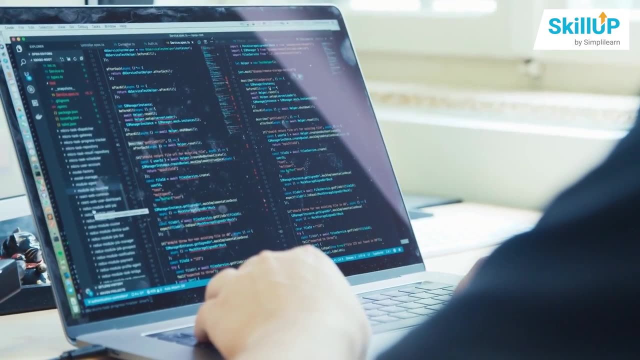 Linux will get you up and running in no time, after which you can check the ethical hackers for beginner courses to further sharpen your skills. Basic scripting skills should be the next step, since developing and combating exploits will require some programming skills. While not mandatory, these scripting skills will help you modify exploits that can later be used to secure. 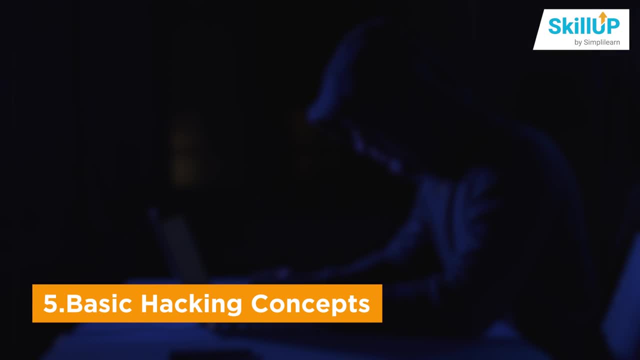 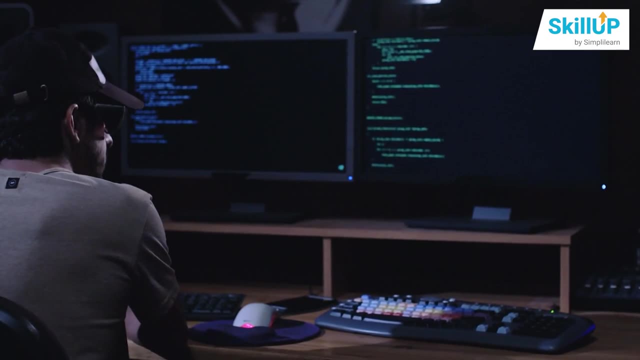 infrastructure. Moving on, you must learn the basics of hacking from scratch before moving on to practice labs or certifications. The Ethical Hacking for Beginners course will cover all the necessary tools to begin your hacking career. You can also learn the basics of hacking from: scratch before moving on to practice labs or certifications. The Ethical Hacking for Beginners course will cover all the necessary tools to begin your hacking career. You can also learn the basics of hacking from scratch before moving on to practice labs or certifications, Thanks to. 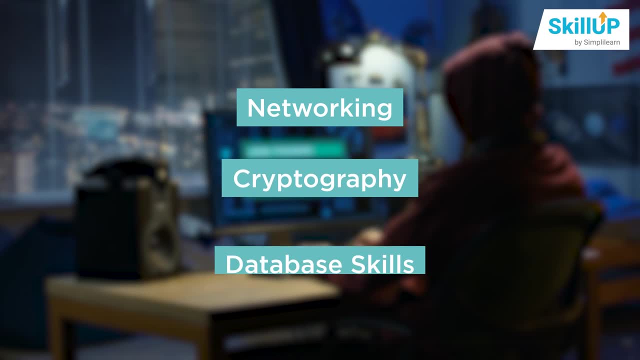 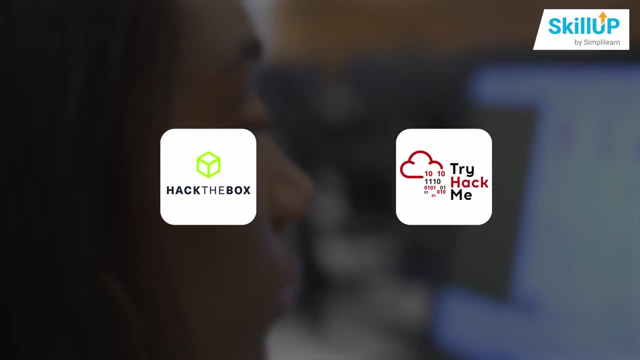 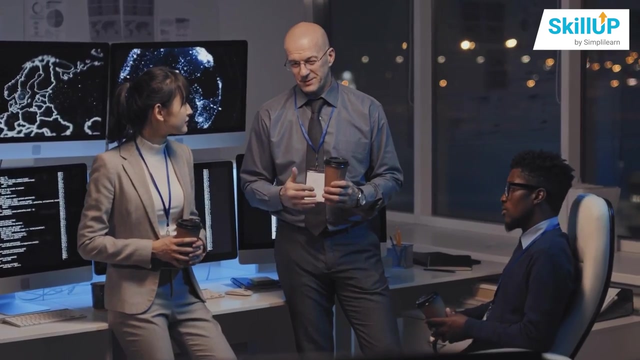 detailed explanations on networking, cryptography and database skills. websites like HackTheBox and TryHackMe are virtual labs that function as targets for ethical hackers practicing their craft As cybersecurity professionals. practicing these rooms can help you stay updated with the latest and most complex tools available to penetration testers today. 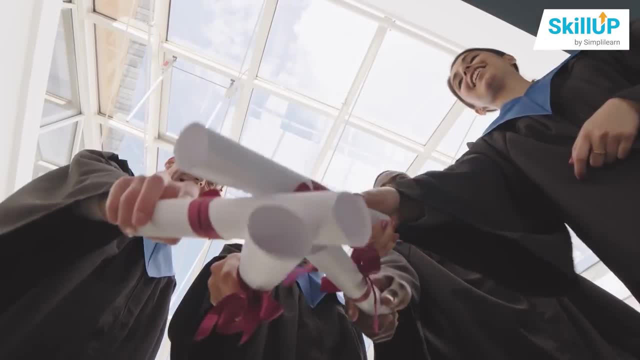 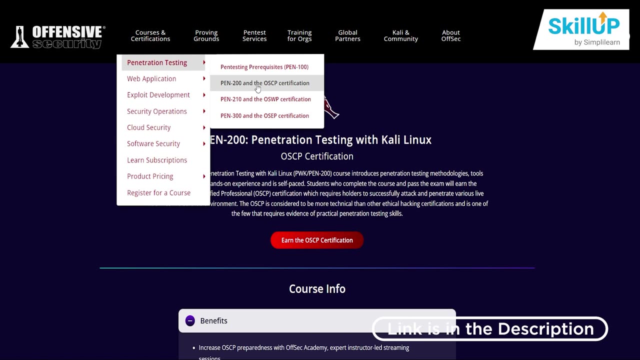 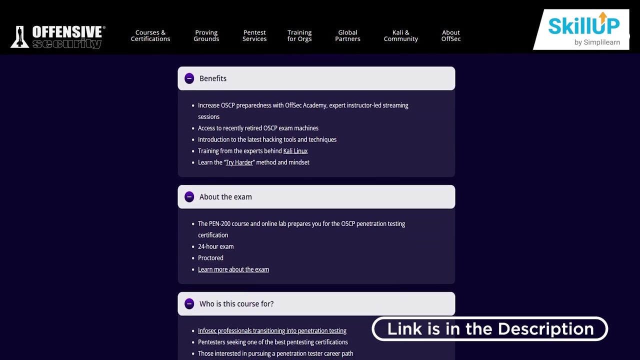 Now regarding a professional certification that can help you grow further in this domain. you have two options. The OSCP online course can be completed at your speed and schedule. It covers penetration testing tools and methodologies through hands-on practice. The program teaches the skills and mindset needed. 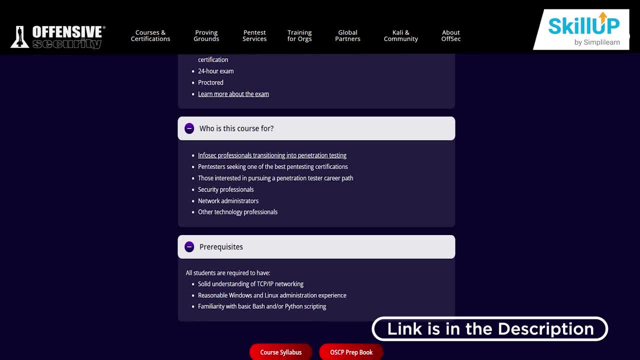 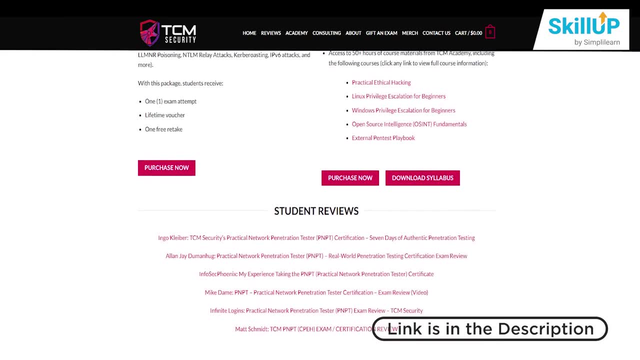 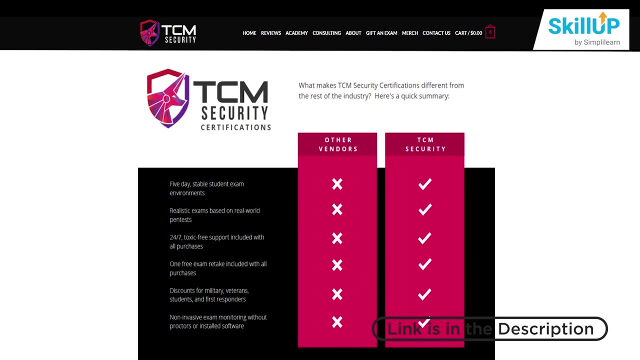 to be a successful vulnerability researcher and a cybersecurity analyst. The PNPT exam, or the Practical Network Penetration Test Certification, is a one-of-a-kind vulnerability scanning certification exam that evaluates a student's capacity to perform a networking penetration test at a professional level. You can thus visit the 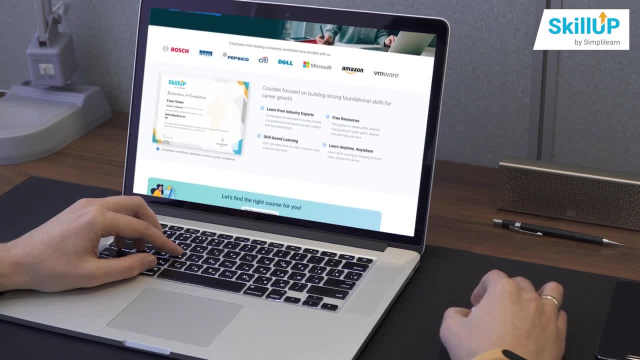 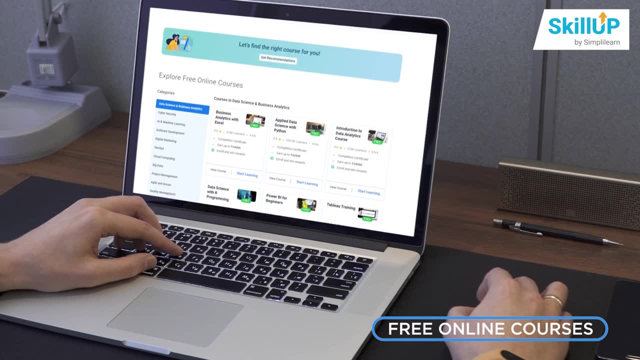 official SkillUp website to learn more about the technologies you're interested in and the free online courses offered there. These courses are self-paced videos taught by subject experts, and you can watch these videos as long as you want and earn a completion certificate at the end of it.